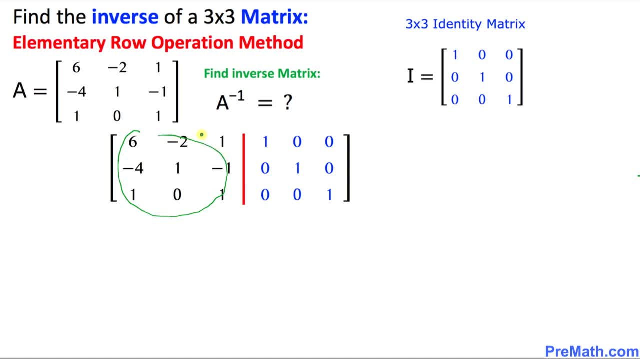 i just put down this one, our matrix A, and, on the right hand side, as you can see, this is our identity matrix. so, in other words, I put down a matrix A on the left hand side and our identity matrix is on the right hand side, and now our job is going to make. 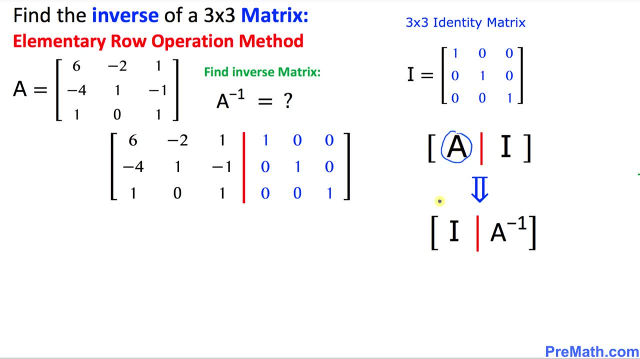 sure that this A is transformed into an identity matrix, then the this, the other matrix on the right hand side, will automatically become an inverse matrix. now let's go ahead and start working on this augmented matrix. so we will be performing this elementary row operation. the very first thing we are to do is 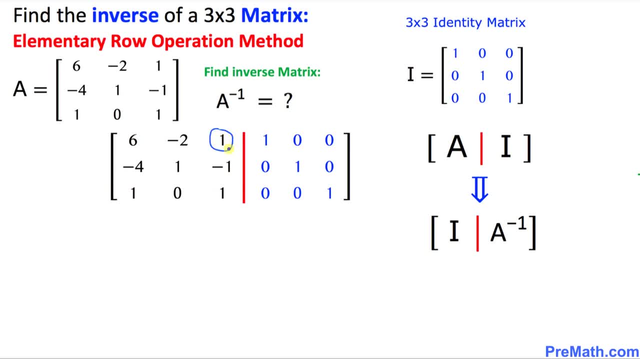 we are. we want to make this 1 and this negative 1. on this row number 1 and row number 2: 0. wherever I put a circle, that means I want to make it a 0. so this is the operation I will be doing. I will be putting down the row 1 minus row 3. 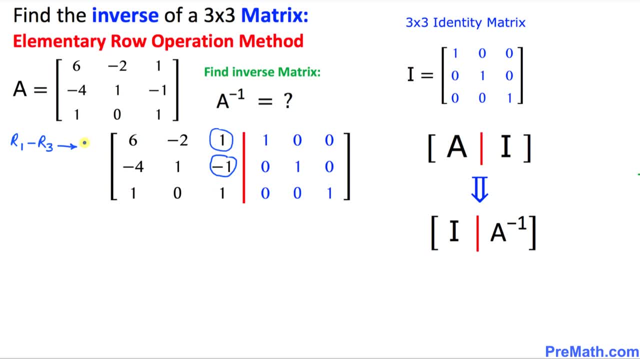 and make sure that I put down the answer in row 1, like that. Likewise, I am going to put down row 2 and then plus row 3.. And once again, the answer is going to go to row 2.. So that's our: row 1 is going to become 5, negative 2, 0, and on this right-hand side is going to become 1, 0, negative 1.. 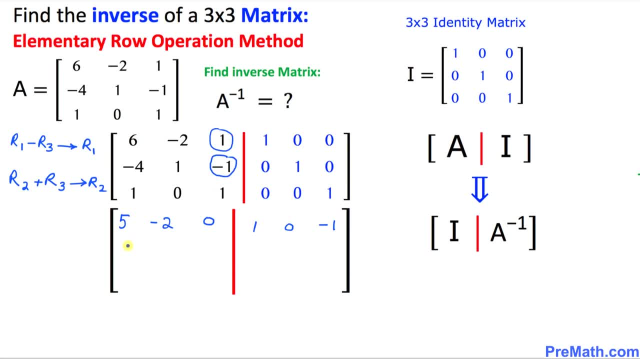 Likewise, we will be looking at the second row as negative- 3, 1.. 0, and on the right-hand side this is going to become 0, 1, 1.. And leave this row, number 3, as it is. We did not perform anything on this one. 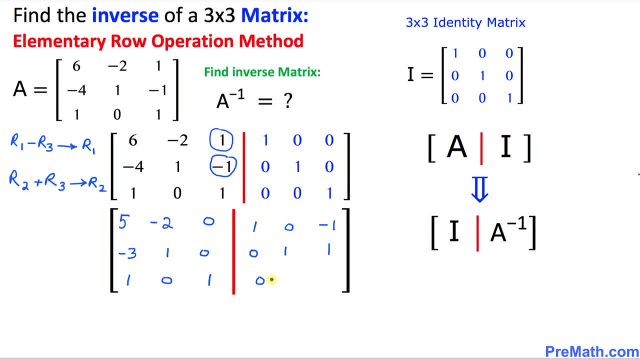 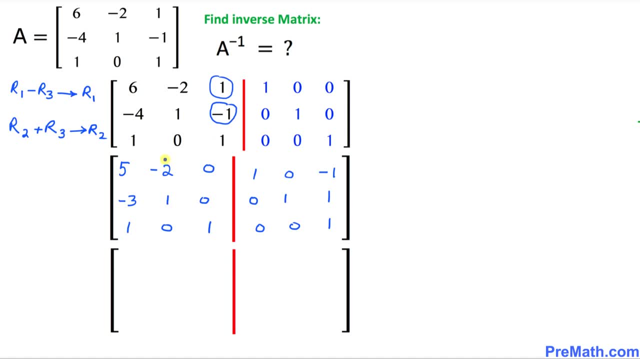 So 1, 0,, 1, and this is going to become 0, 0, 1.. And now, in the next step, we are going to make this negative: 2. In the first row, 0. To do that one, we are going to put down row 1, r1, plus 2 times row 2, and then put the answer in row 1.. 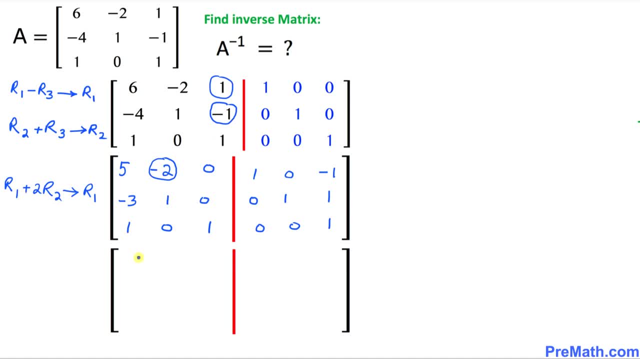 So then we will get this become: first row is going to become negative: 1.. 1,, 0,, 0, and on the right-hand side, this is simply become 1,, 2,, 1.. And the other rows are going to stay the same. 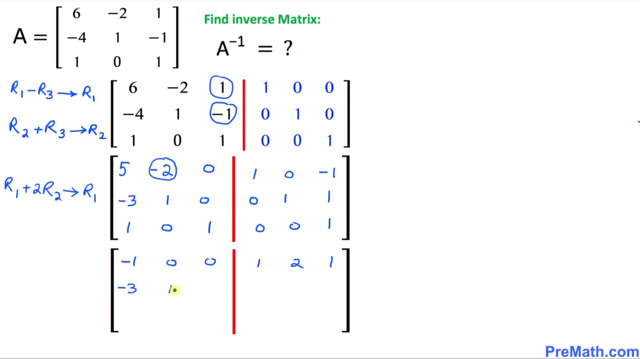 So I'm going to just put down negative 3, 1, 0, 0, 1, 1.. And likewise 1, 0.. 0, 1, 0, 0, 1.. 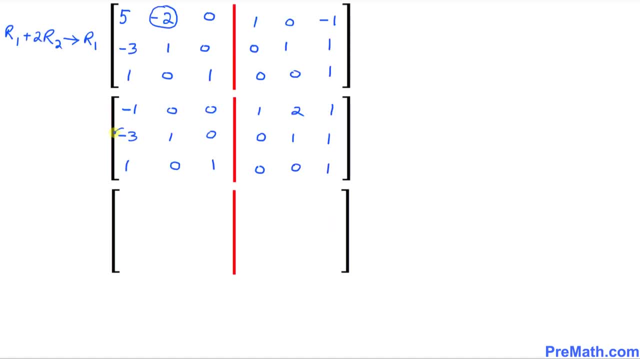 And now we are going to make these negative 3 and 1 in row number 2 and 3 zeros. So for that one I am going to do these operations. So I'm going to say row 2, minus 3, row 1.. 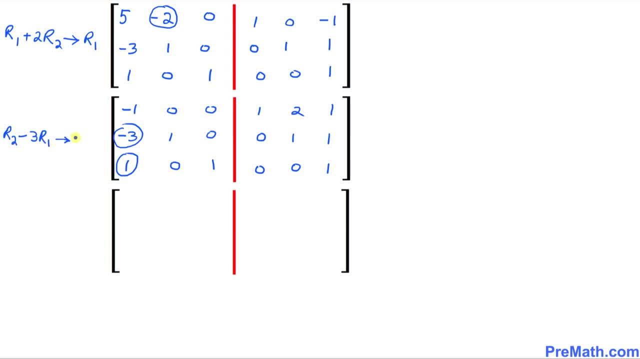 And put the answer in row 2.. And for row number 3, I am going to say row 3, plus row 1. And put down the answer in row 3.. For that one we are going to get negative 1.. 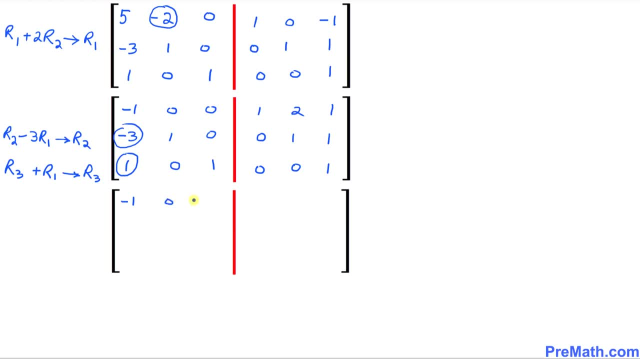 Negative: 1.. The first top row is going to stay Same, isn't it So? 1, negative. 1, 0, 0.. And this is 1, 2, 1.. The second row is going to become 0, 1, 0.. 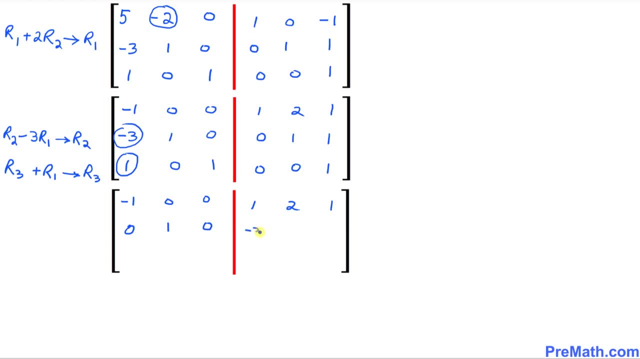 And here this is going to become negative 3, negative 5,, negative, 2.. And finally, in row, number 3.. We are going to get 0, 0, 1.. And this side is going to become 1,, 2,, 2.. 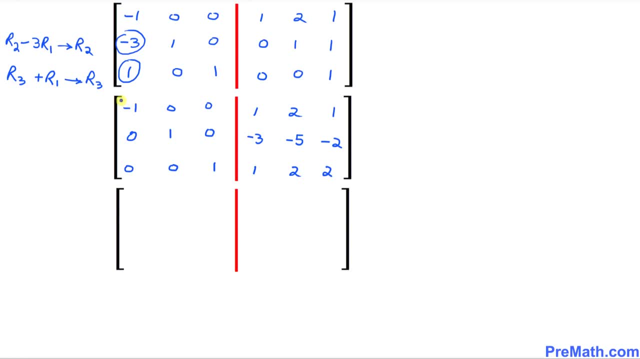 And now we are almost finished. The only thing we can see that this negative 1, we want to make it a positive 1.. So we are going to multiply the row 1 by negative 1.. That's all we do. 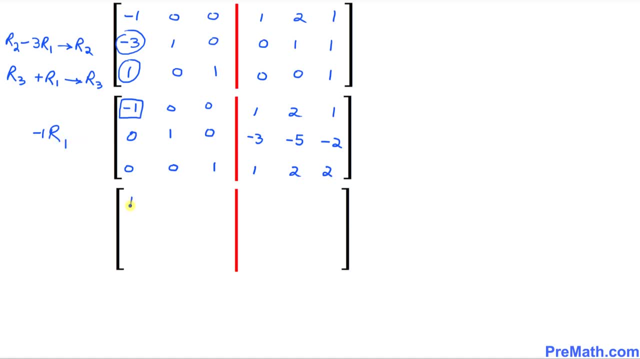 Negative 1 times row 1.. So that is going to become 1, 0, 0.. And on the right hand side, this becomes negative 1, negative, 2, negative 1.. The rest is going to stay the same. 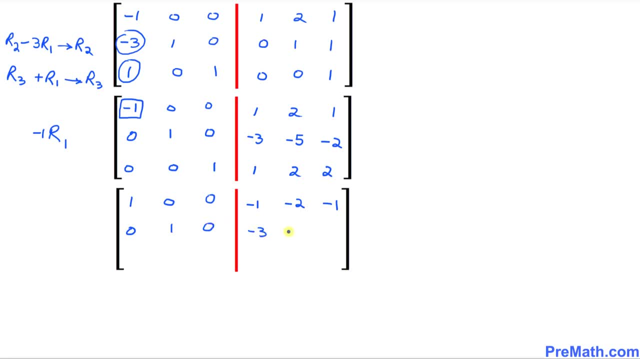 0, 1, 0, negative, 3, negative 5, negative, 2.. And finally, 0, 0,, 1,, 1,, 2,, 2.. And now, as you can see, our left hand side matrix has been transformed into an identity matrix. 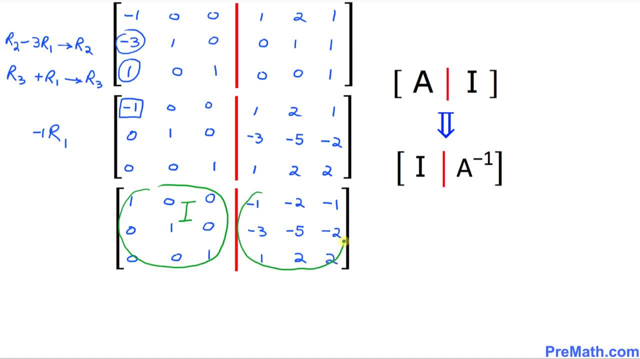 So then, this right hand side matrix will be automatically A inverse matrix According to this, our, this given rule. Thus, our A inverse is our inverse matrix, and that is our answer. And here is your assignment. Can you do this problem on your own now? 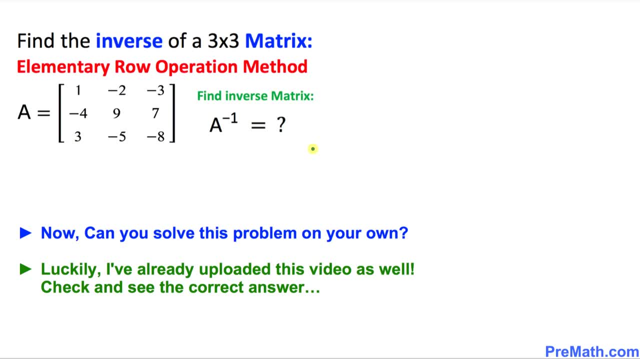 You can take your time. You can pause the video. Luckily, I have already uploaded this video as well. Please go ahead and check it out and see the correct answer, Thank you. Thanks for watching and please don't forget to subscribe to my channel for more exciting. videos Bye.